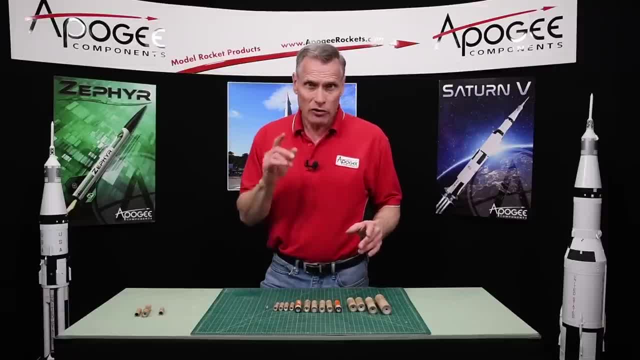 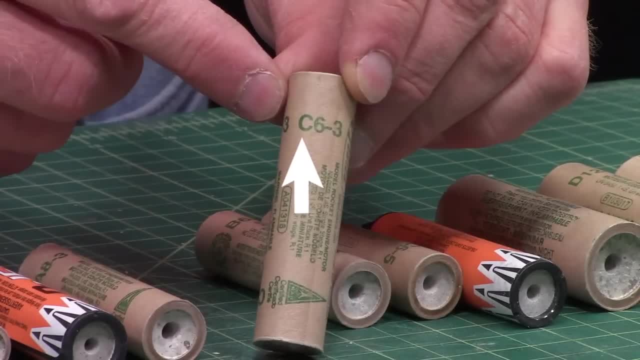 for your rocket. Well, I'm going to try to explain that. The first letter say: here on this rocket, right here I have a C63.. This letter tells us the relative power of the motor. In rocketry we use A. 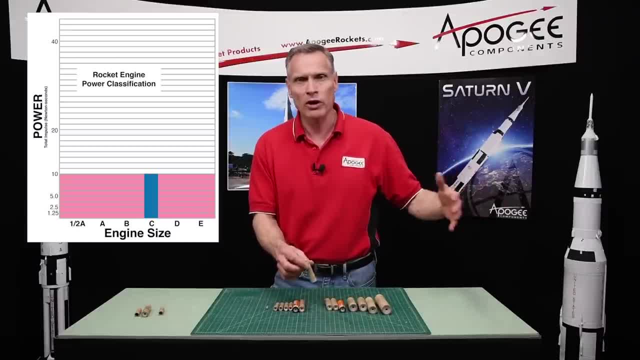 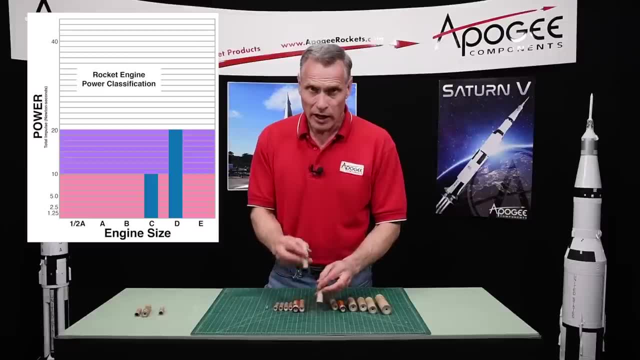 B, C, D, the letters of the alphabet to explain power. So whenever you go from one letter to the next, it doubles in power. Whenever you go from one letter to the next, it doubles in power. So a B motor has half the power of a C motor. This is a B motor And the way they do that. 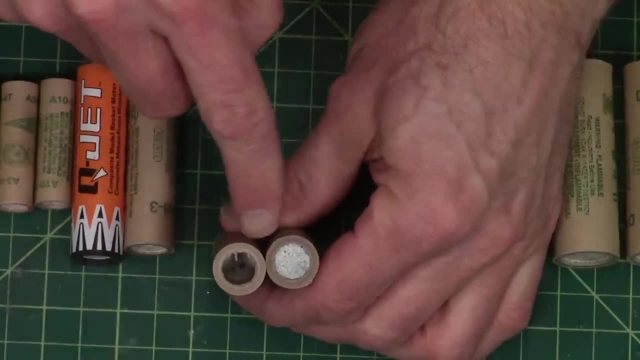 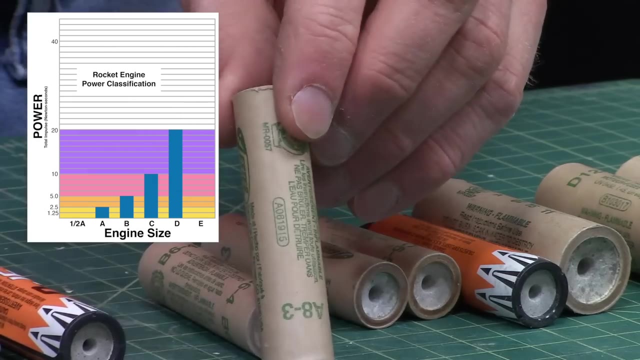 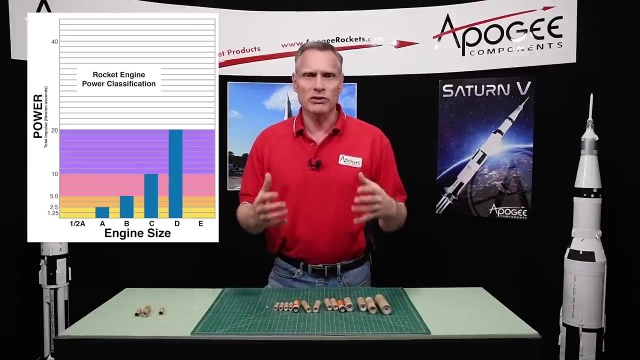 is by filling it up to a different level inside the rocket. Now they can go down, so an A motor has half the power of a B motor or one quarter the power of a C motor. So what this really means is if your A motor, if your rocket with an A motor, goes approximately 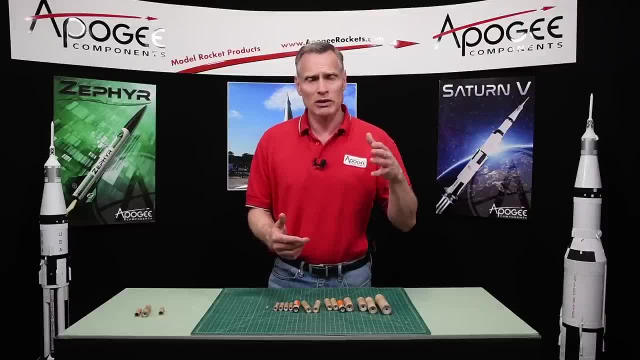 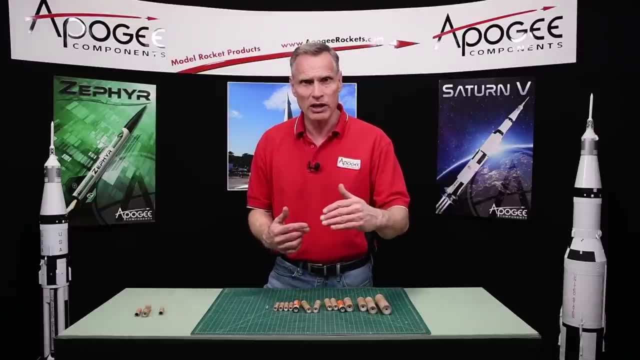 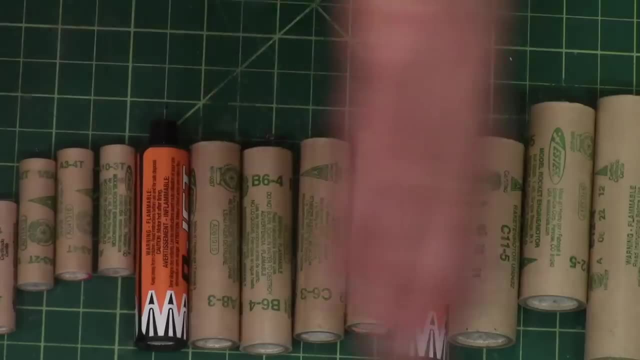 one hundred feet. if you put a B motor in it it will approximately go two hundred feet. It doubles in power. you can go twice the distance A C motor is going to go twice that of a B- about four hundred feet in a given particular rocket. Here on the table I have a variety of rockets, from the smallest. 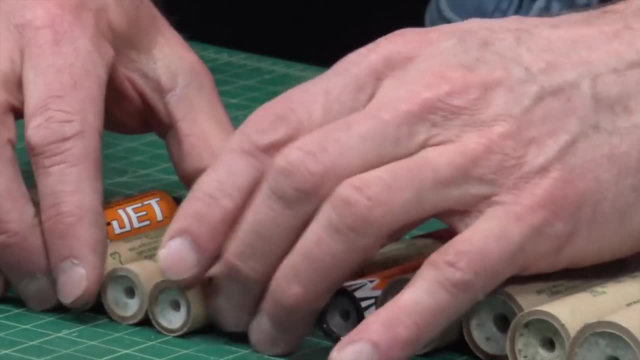 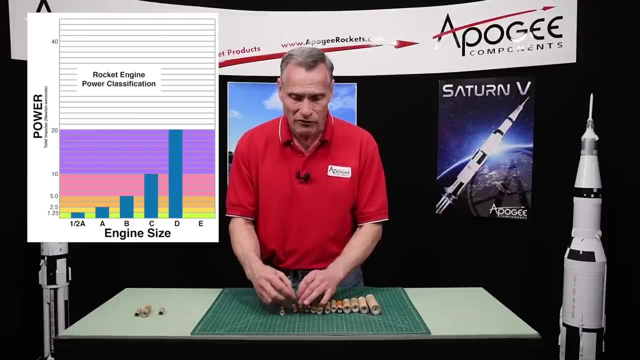 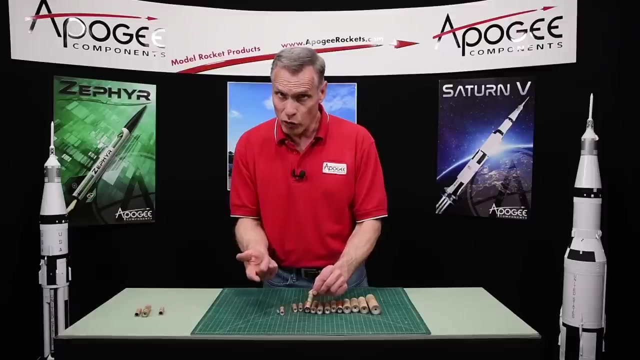 to the largest. So I already had As B's and C's which are right here. You can go smaller than that. smaller than an A would be a half of an A and this motor right here is labeled half A. You can go half of that again as well. 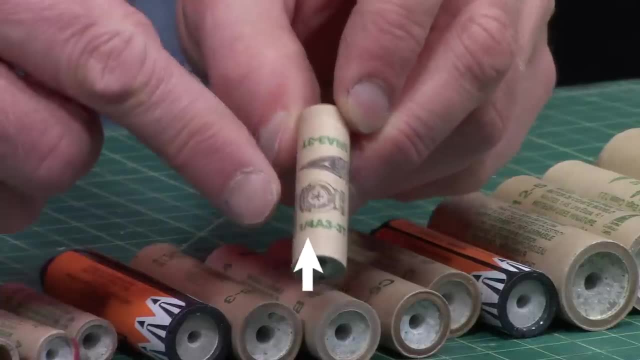 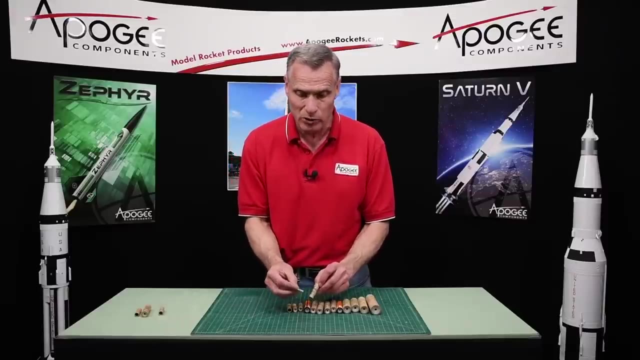 And so this small motor is a one quarter A, And then half of that, which is the smallest motor available in rocketry, is an eighth of an A, And these are pretty much for variety and for very, very small launch areas like a backyard. 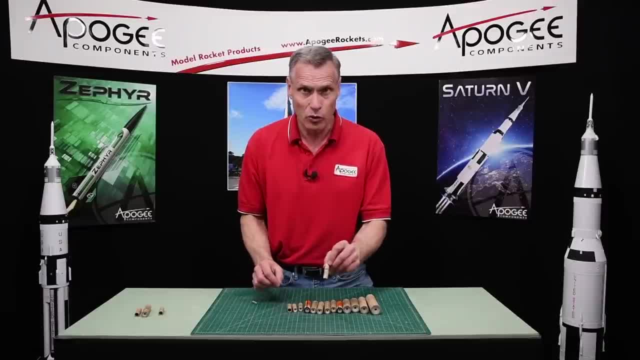 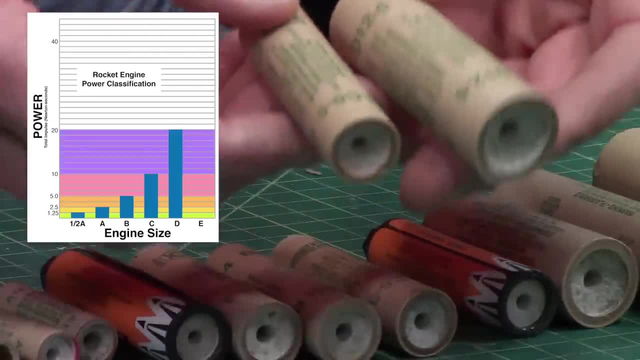 But typically in model rocketry the smallest that we use is a quarter A And then it goes up. from there You can go a D, which is twice as powerful as the C motor, And again they filled the casing all the way up. 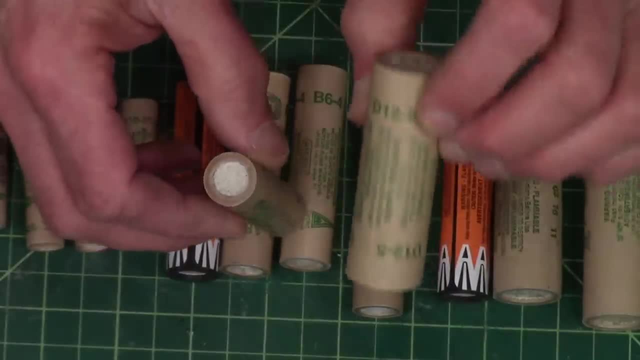 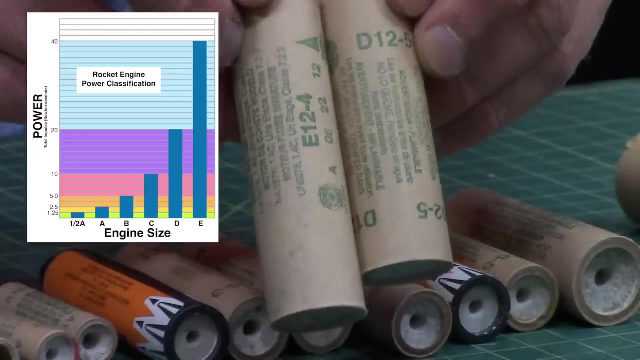 but in order to get twice the propellant inside, they had to go to a larger diameter. And then there's the E motor Which again, compared to the D motor is a lot longer. And then the F motor is even longer still. 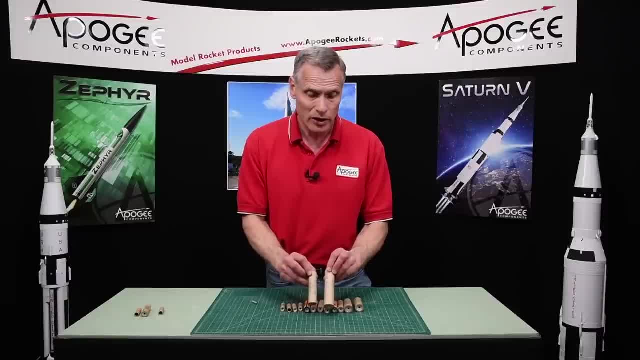 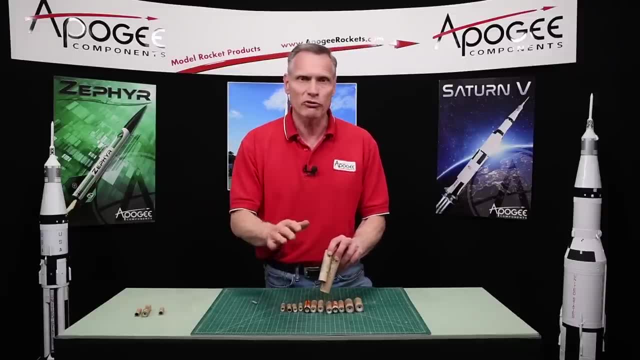 And the F motor is about the biggest you'll find in a black powder motor. But you can go higher than that to a G motor in composite propellant, which is a different propellant which will be for a different video. So that's the first letter. 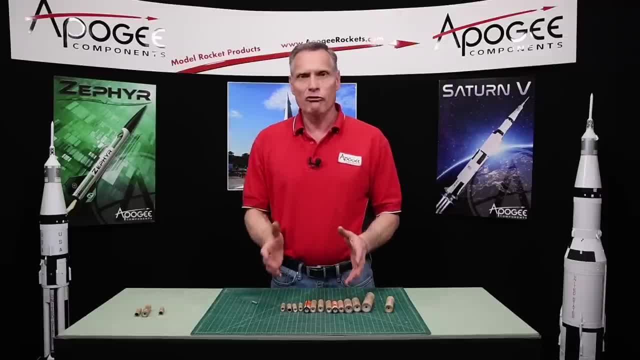 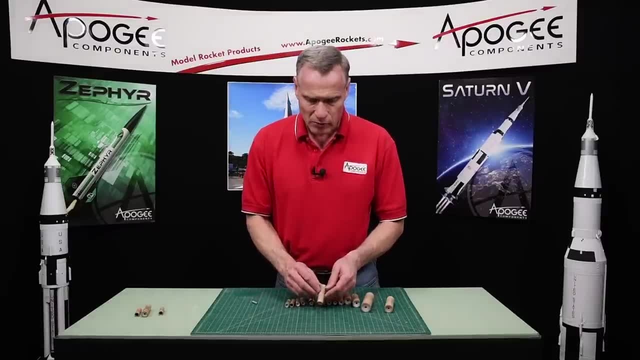 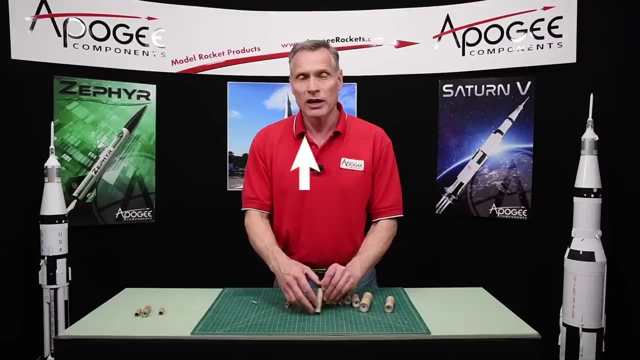 The first number indicates the average thrust of a rocket motor And it's measured in newtons. So this rocket motor right here is an A83, so it has an average thrust of eight newtons. Now, when you go to pick motors, 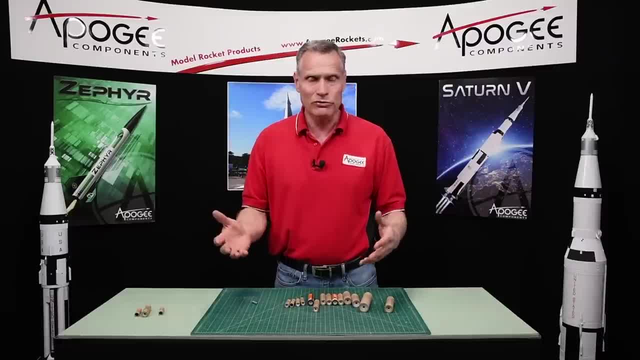 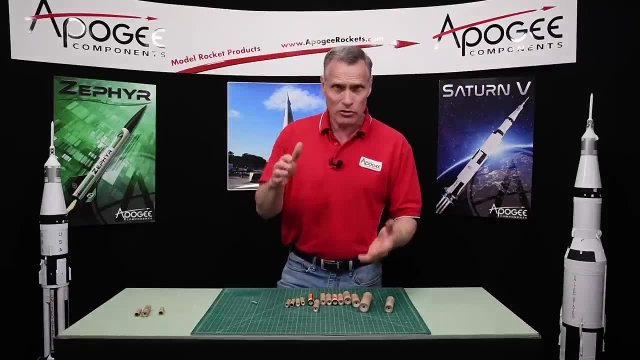 you're not going to say: I need a rocket that has exactly eight newtons or nine newtons or 10 newtons. it's a relative number. The bigger the number, the higher the thrust. The smaller the number, the lower the thrust. 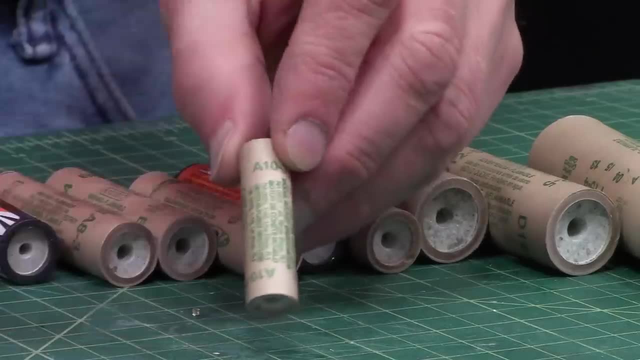 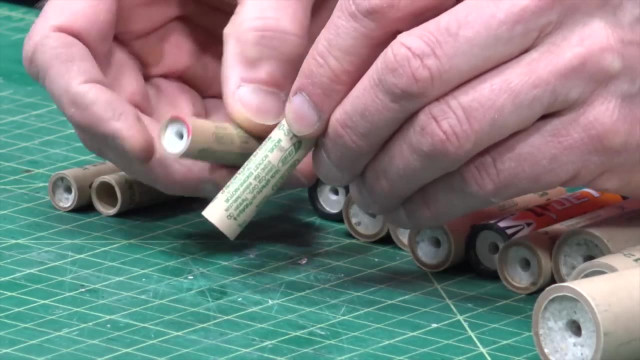 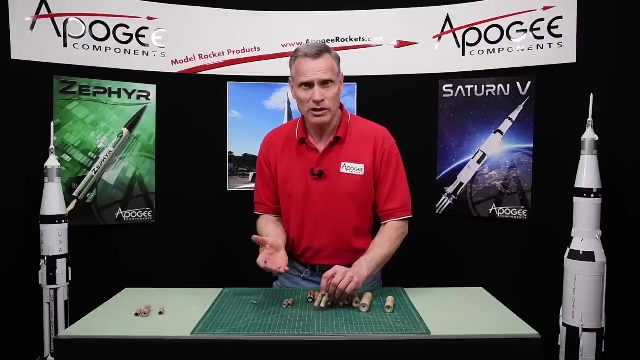 So here is an A10. And now we have to measure this, So it has an average thrust of 10 Newtons. And then, next to it, here's an A3.. They're going to go approximately the same height, approximately, but this is where aerodynamics 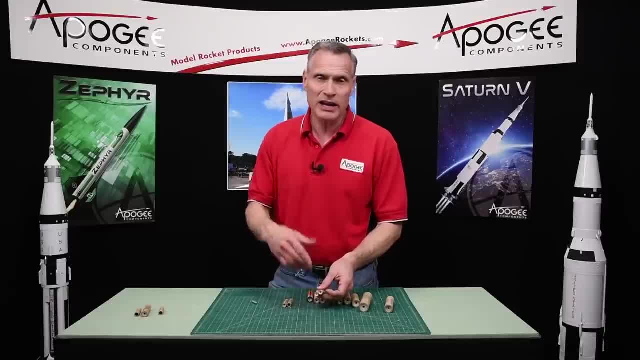 plays a role. An A10, what it means is it's got a higher thrust, so the rocket's going to take off faster than the A3. So think of it as how much pressure you're putting on the accelerator pedal of your car. 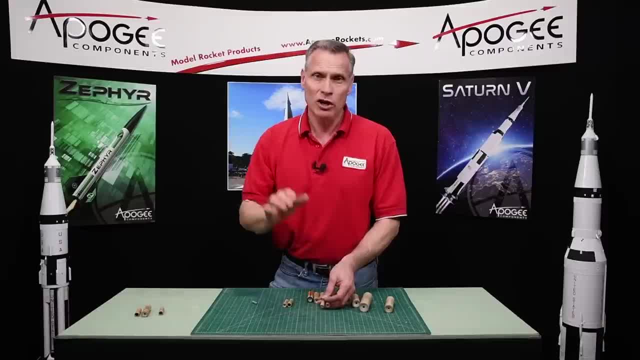 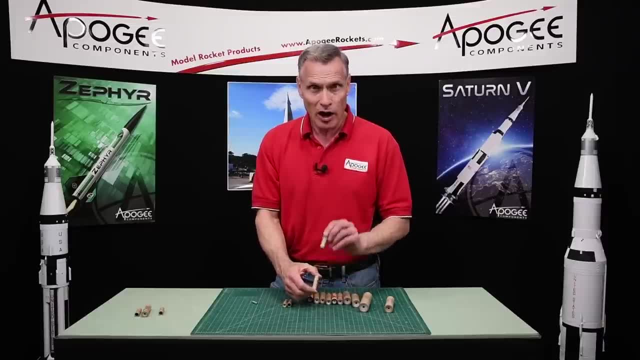 If you push down just a little bit, you're going to take off nice and slow. If you stomp on it, you're going to accelerate really fast. So if you want to go fast, use a higher number, and if you want to go slow, use a lower number. 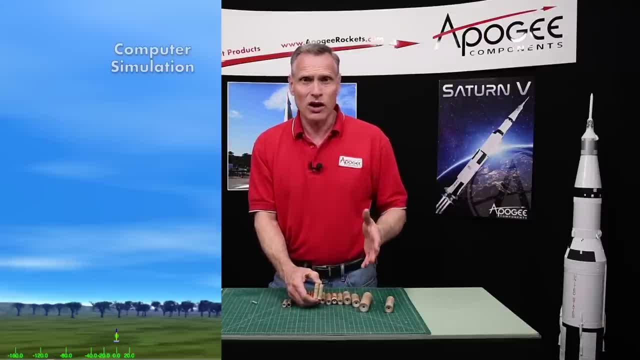 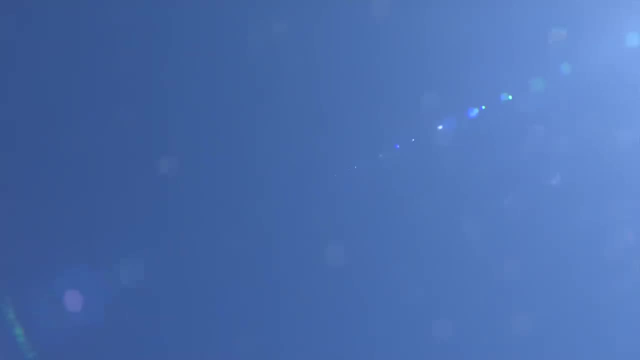 Also, when the rocket takes off because it's going slower, it's going to weathercock a little bit. So here's a video of two rockets taking off, and I tried to get them to take off exactly at the same time, but one of the igniters took a little bit longer to heat up. 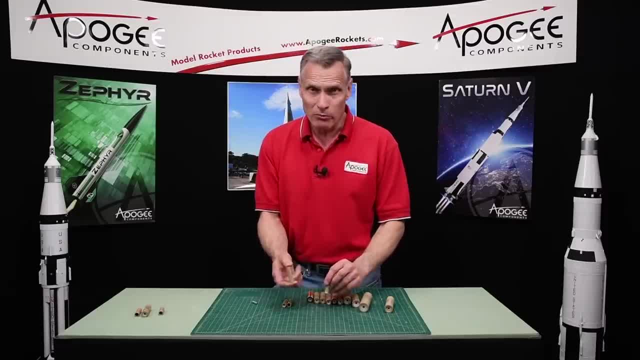 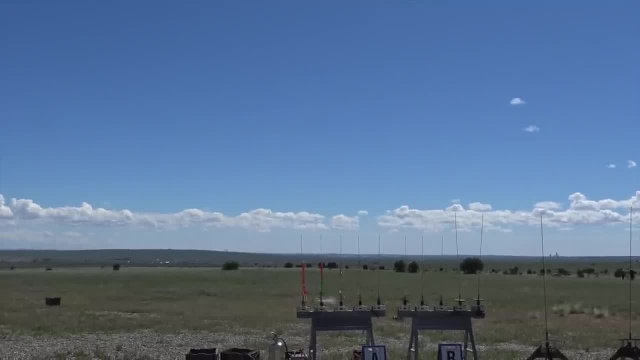 So don't think that a smaller number means that it's going to take off slower when you push the button. That's not the case. It just happened. this igniter didn't take off like right away, like the other motor, the A10.. 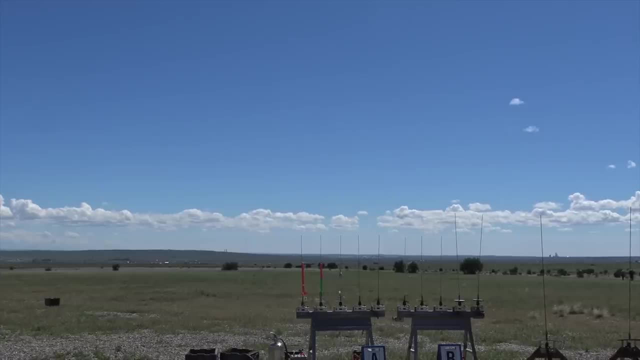 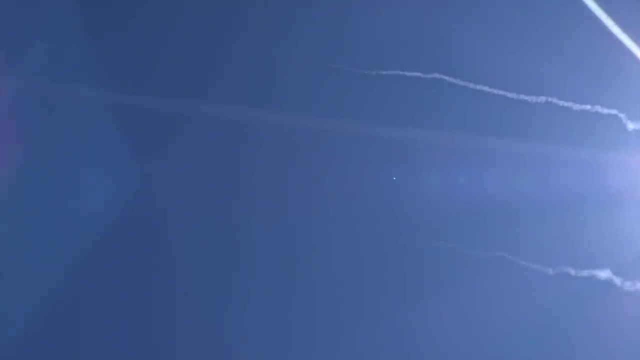 But notice the trajectory of the rockets. The A10 took off first and it went fairly slow. It went fairly straight, but the A3 started weathercocking into the wind. So you have to remember that when you take off slower you're going to weathercock a. 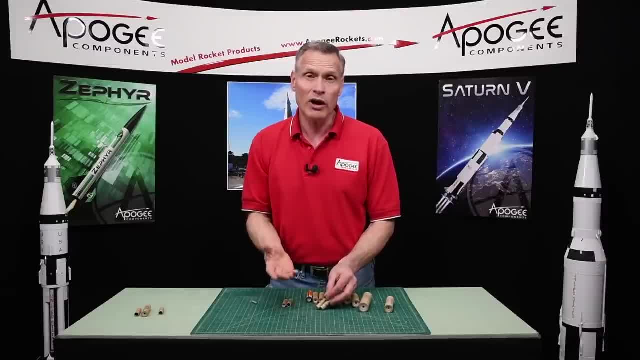 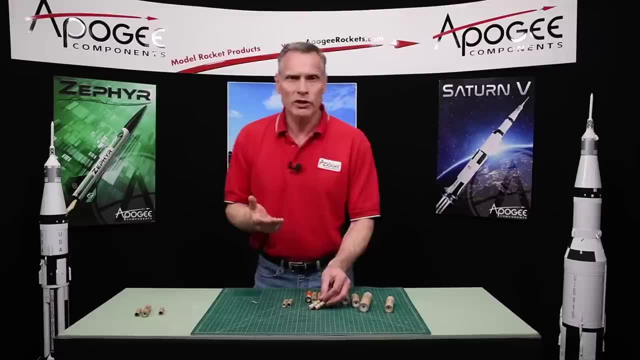 little bit more. If you have a windy day, you probably want a higher thrust motor, and if it's a nice calm day you can go with a lower thrust motor. The other thing about a lower thrust motor is because you're traveling slower. the drag. 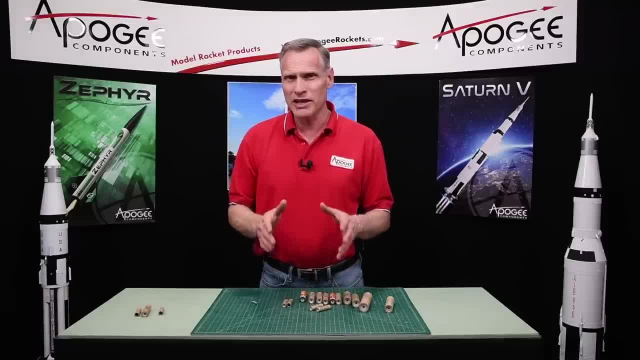 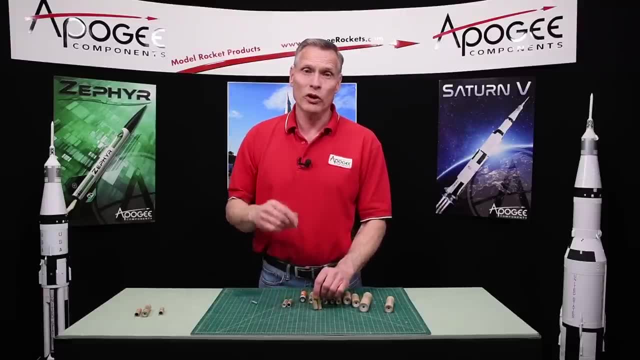 on the rocket is lower. What this actually means is that the lower thrust is actually going to go a little bit higher than the one with higher thrust. So if you want to go high, choose a motor that has low thrust, but if it's windy you're. 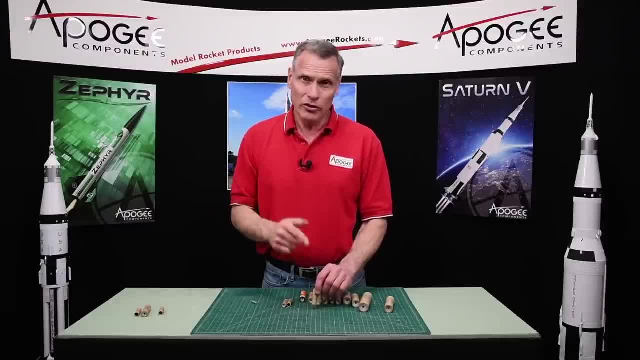 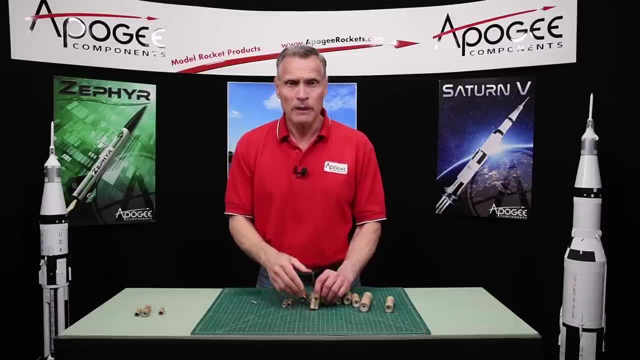 going to lose a lot of altitude because it's weathercocking into the wind. So in that case you might want to go with the higher thrust motor. Again, this is relative, so you have to look at the motors that you have available and 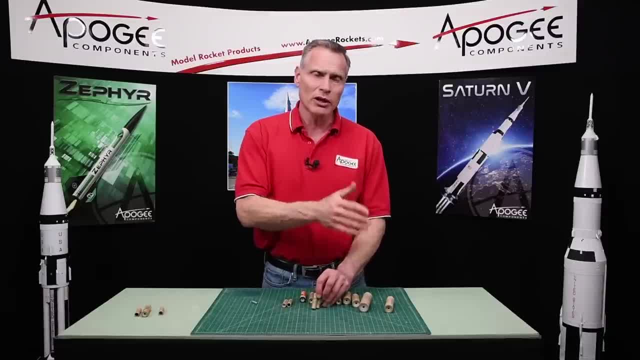 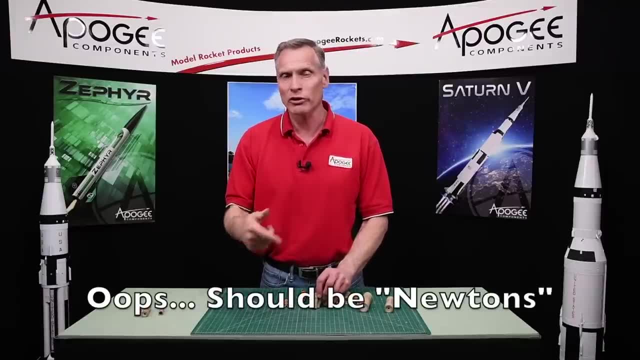 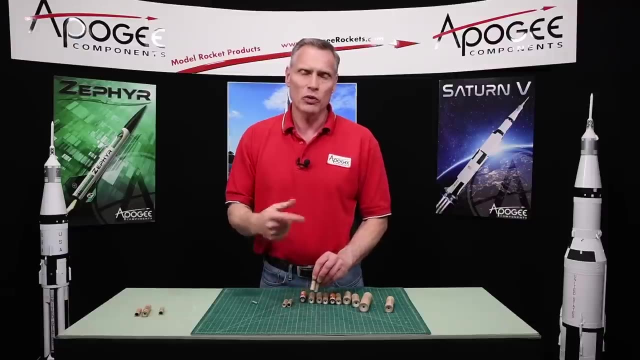 then choose from that. So you don't say I need a three-second average thrust motor. No, you say I need a three-second average thrust motor. Okay, What's the launch conditions today? Is it going to be calm? Then I'm going to use a low thrust motor, and if it's windy, I want to use a high thrust. motor. Or if my rocket is heavy now I need more oomph to get it going. This is called inertia. When you're pushing like a car, it takes a lot of effort to get it to move because it's heavy. but once it's moving then you can sustain it pretty good. 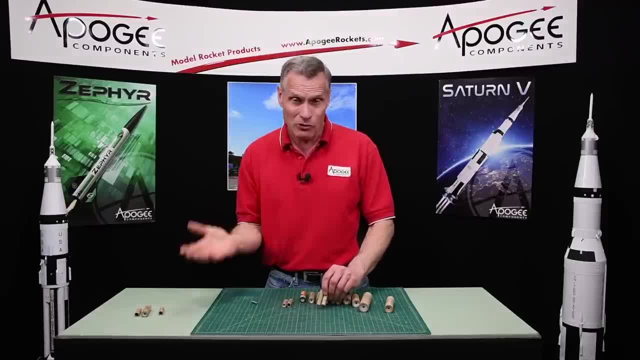 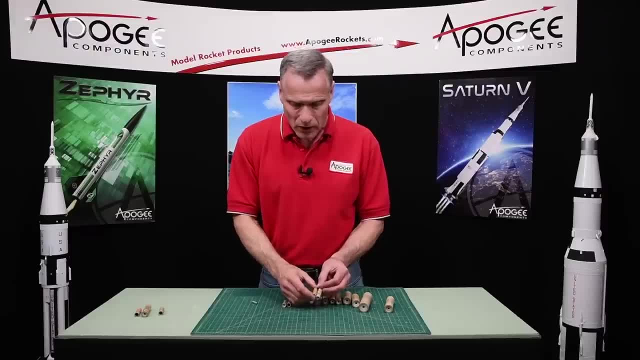 So when the rocket takes off, you want on a big, heavy rocket, you want a high thrust, Okay, You want a high thrust to get it moving and then it will travel. nice, Okay. so now that's the first number in the code. 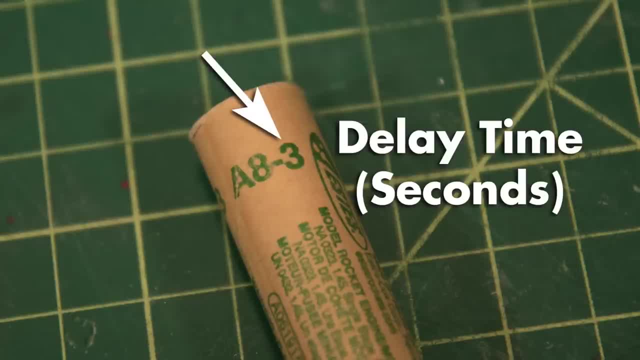 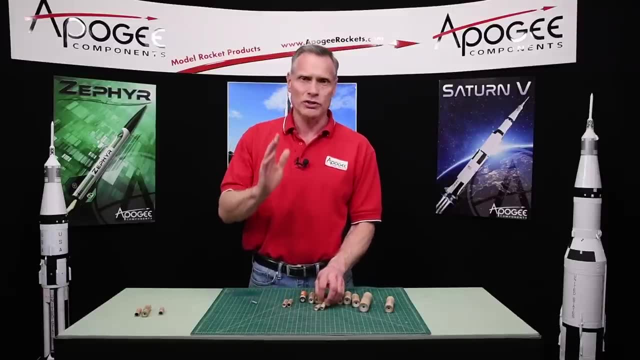 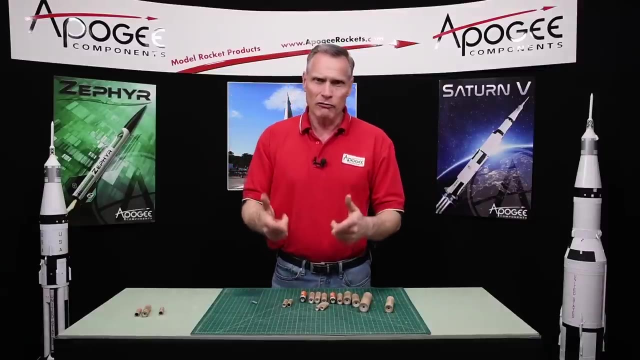 The second number, which is always after the dash, is the delay in seconds. It's measured in seconds And this allows the rocket to coast. Because what happens when the rocket takes off? it burns its propellant and the highest velocity of the rocket. The rocket is right about when the rocket burns out, when it consumes all the propellant inside the motor casing. At that point the rocket could be going over 200 miles an hour. But you do not want to kick out your parachute at that point because it's going to just 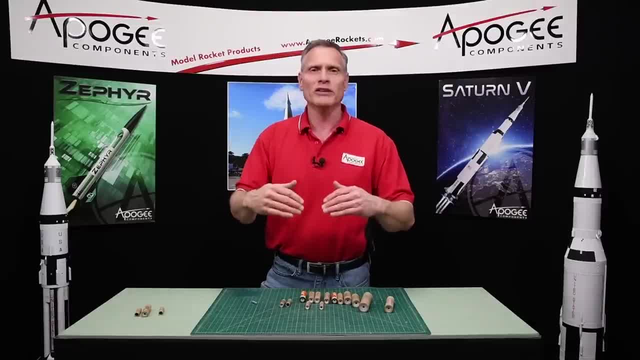 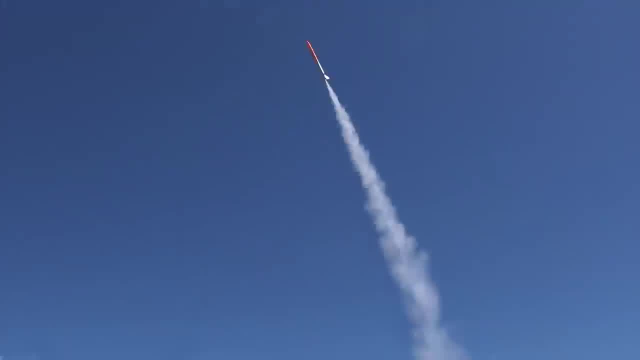 shred the parachute So we want the rocket to coast, We want it to slow down, so that when we do push out the parachute it's at a nice slow speed and the parachute survives And also the rocket can coast. It can coast higher into the air. 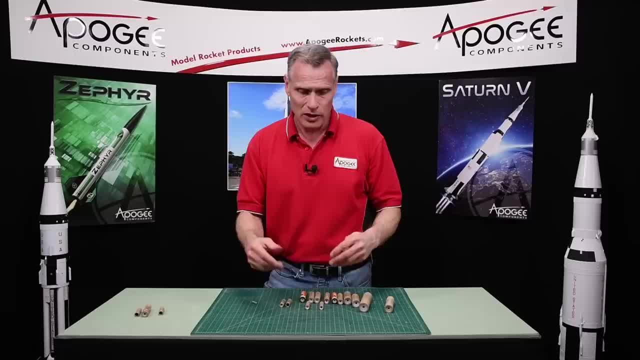 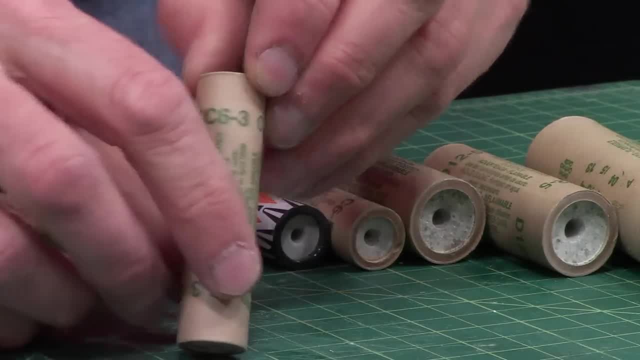 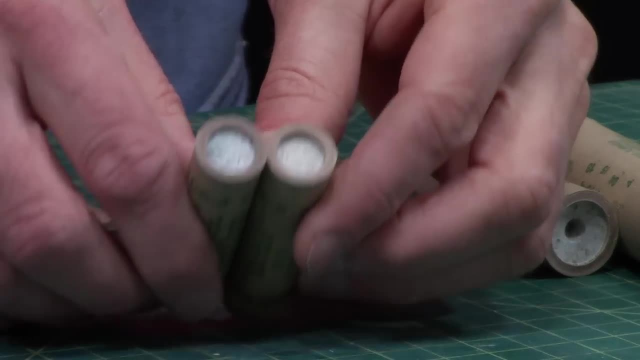 So that last one tells us how long it's going to coast. So here I have a C-6-3, and then next to it I have a C-6-5. So these are both C-6 motors and they have about the same amount of propellant in it. 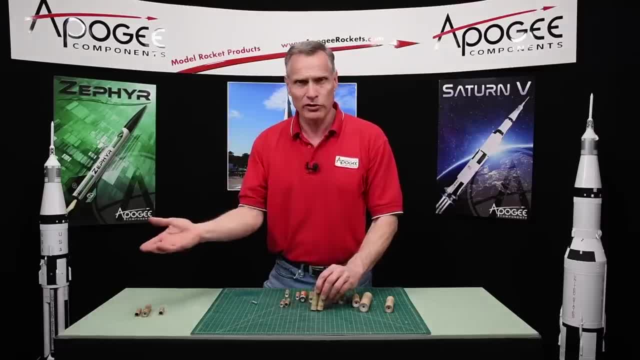 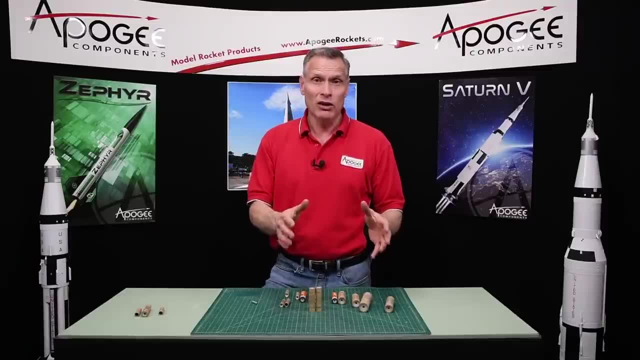 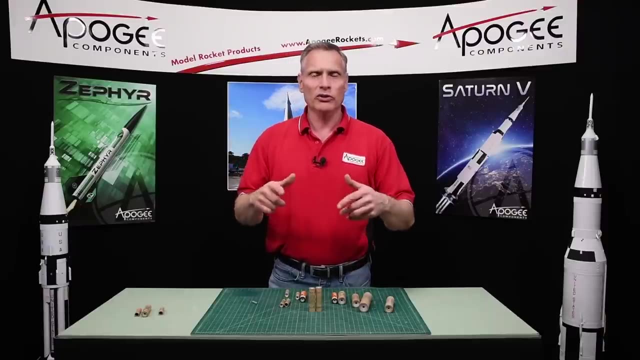 But the C-6-3 is going to eject earlier in the flight than the C-6-5. Sometimes that can be good, sometimes that can be bad. So here's what you want to consider. So if your rocket is lightweight, you want it to coast longer. 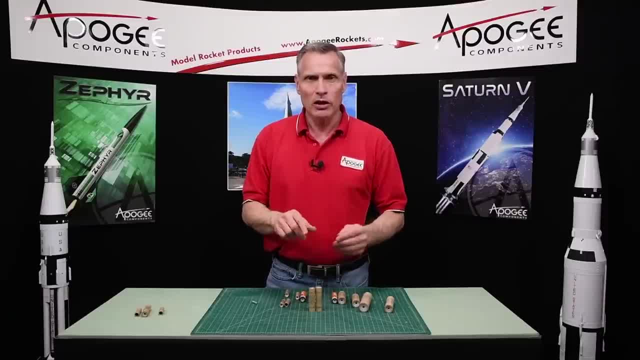 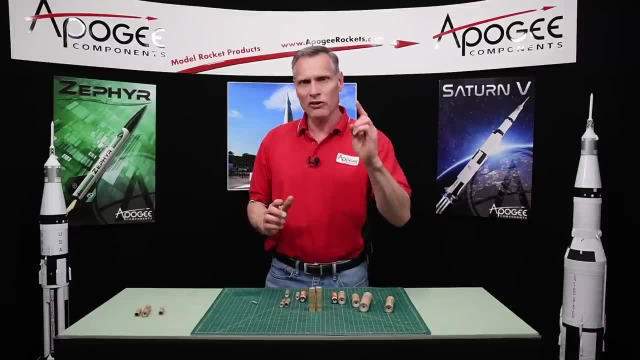 If it's a heavier rocket, you want to use a shorter delay. Also, if it's windy, you might want to use a shorter delay, because what's going to happen on a windy day? Your rocket is going to take off and it's going to arc into the wind and it's not going. 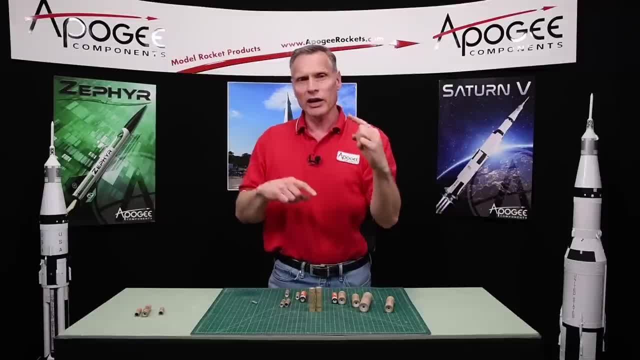 to go as high. It's going to go this way. So the amount of delay is going to be lower because you're not coasting as high. So that's what you want to consider. So on a windy day, shorter delay. On a calm day, a little bit longer delay will be okay. 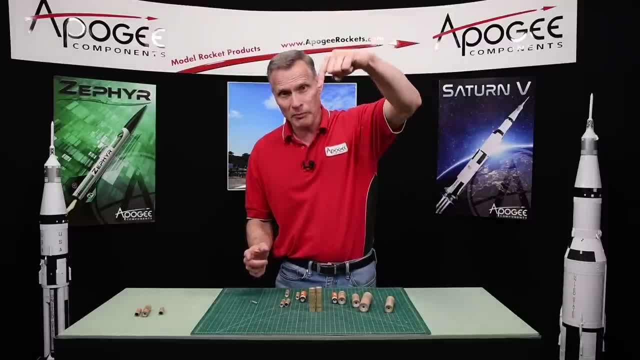 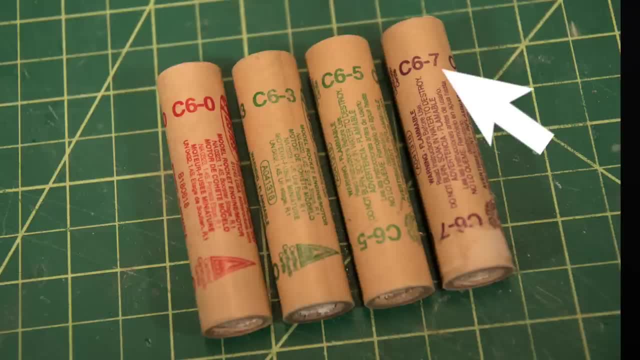 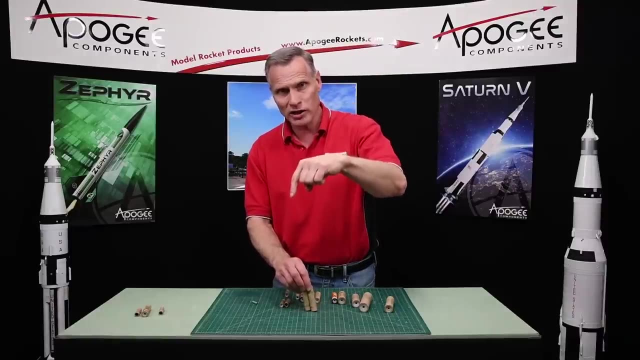 If you go too long the rocket can come over the top and be coming back down when the parachute is ejected. So there's another motor called a C-6-7.. It has a seven second delay, which is really long, And typically those will come over the top and eject on the way down. 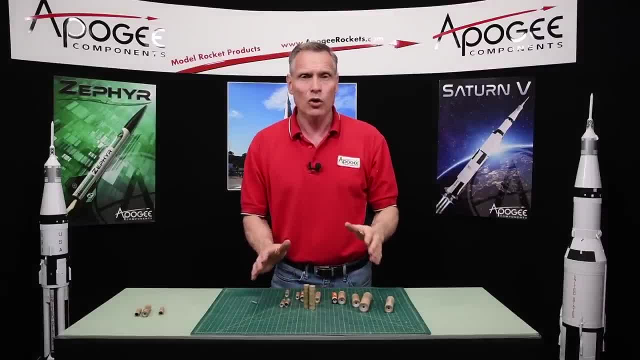 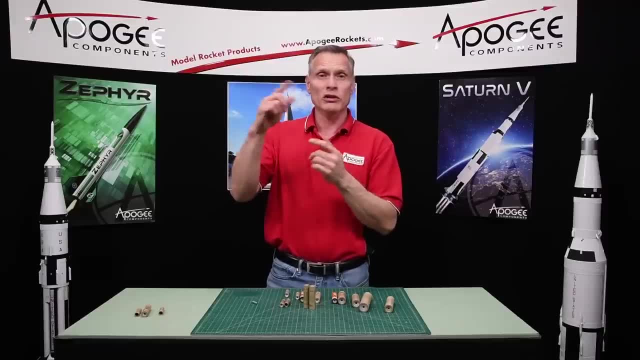 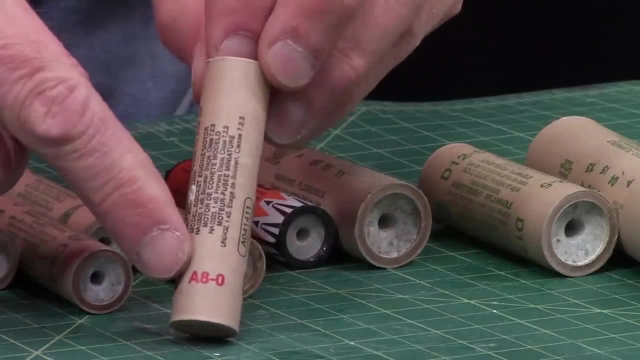 So those are good for really, really lightweight rockets. And then there are more rockets that are two-stage. On a two-stage rocket you have two motors pushing, and so you can coast a lot further. So if you have a motor that has a zero on it, like this one right here, this is an AA-0.. 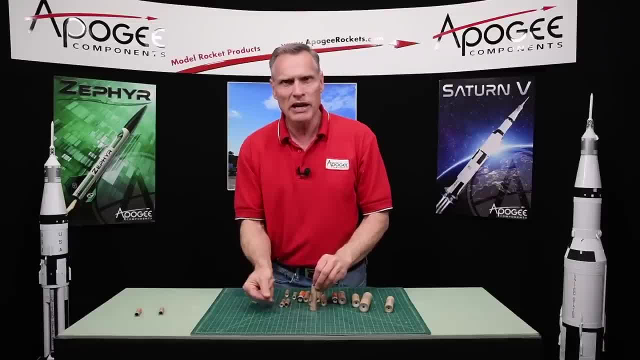 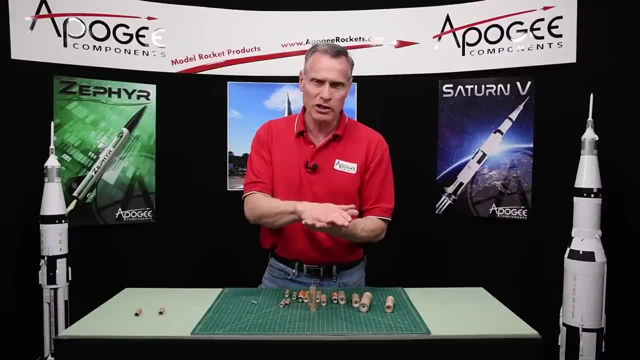 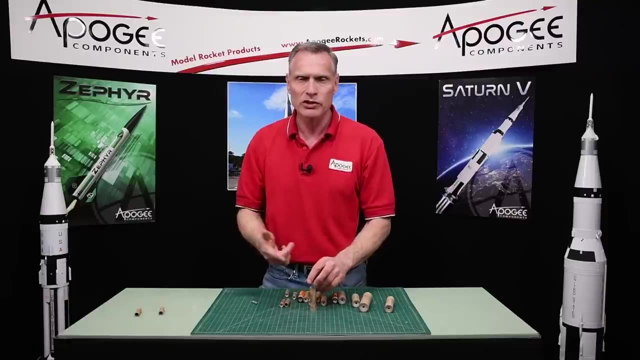 That means that the ejection charge will fire immediately after the propellant is consumed. So that's the starting point. When the motor is done consuming the propellant, that's when the delay starts. So if it's a zero second delay, it immediately kicks out the ejection charge.